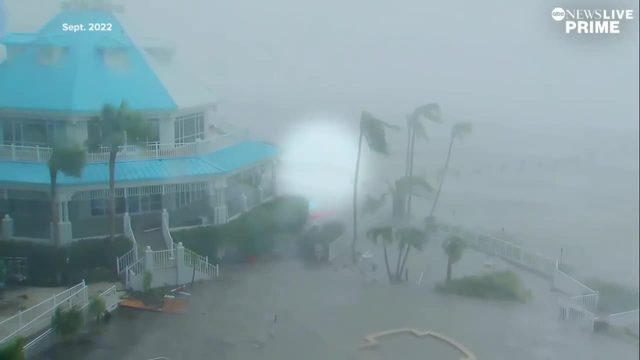 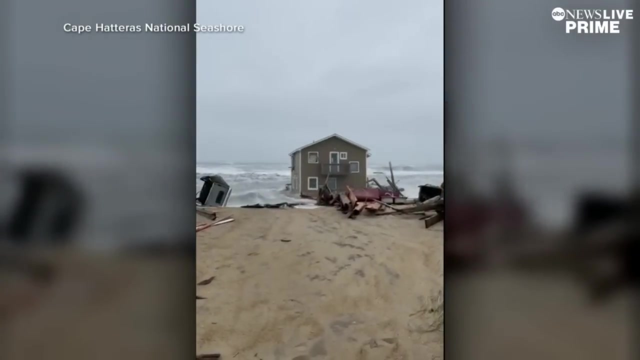 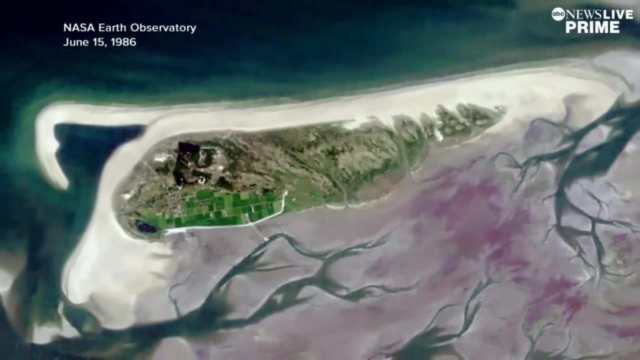 Succumbed to the storm surge. Now the blue roof is all that's left, floating in the water toward the building. Erosion is part of Earth's natural cycle and an increasing reality in some of the country's most visited beaches. Human-induced climate change has amplified the pace of rising sea levels, which magnifies the pace of erosion. 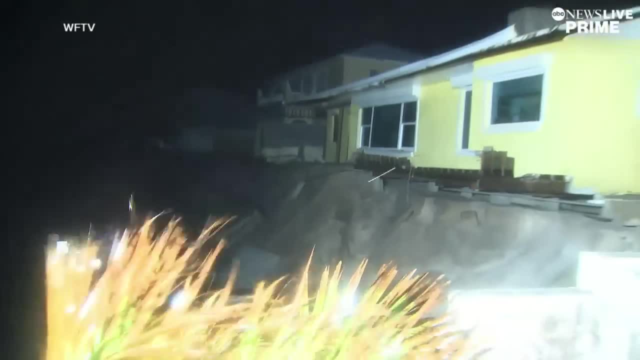 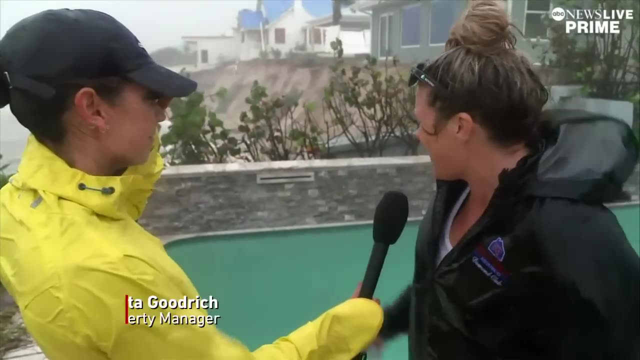 It also increases the amount of water in the ocean. It all happens faster when supercharged storms repetitively gnawed the beaches. It has been a very difficult year for us. We are surprised that we normally don't get hurricanes here And now we've gotten two pretty strong ones, so it's been shocking for us. 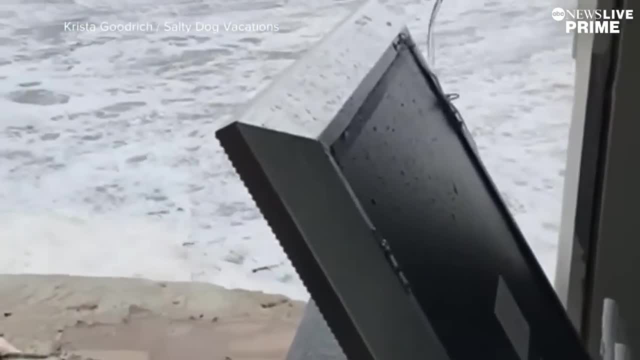 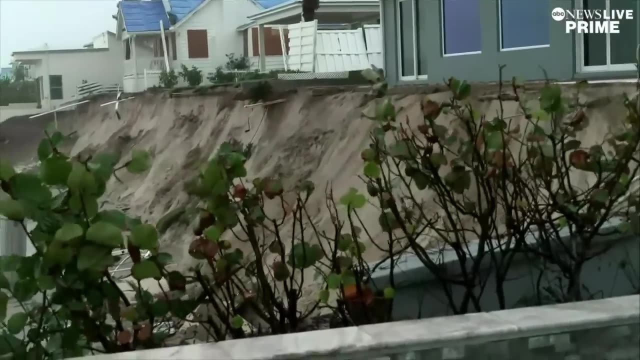 Krista Goodrich is the property manager for several homes in Daytona Beach. She watched her coast disintegrate in just 44 days. Yesterday this property right here had a backyard about 30 feet. We lost 30 feet for Ian, but then the rest of it collapsed. this morning 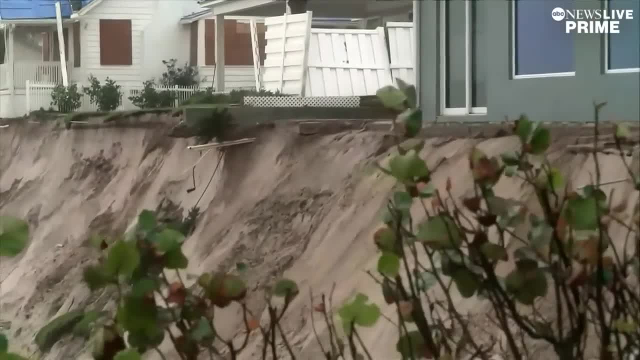 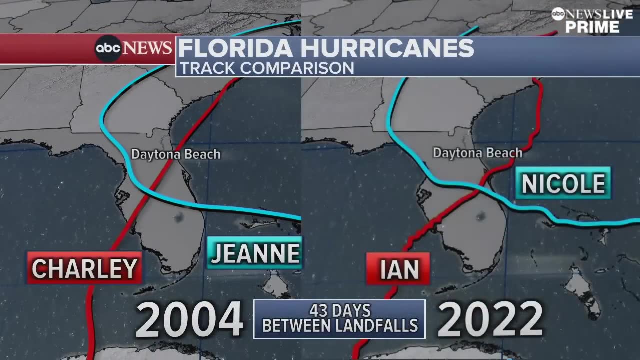 While we were evacuating the owner, as we were moving furniture to get it away from the back of the house, we were watching the backyard just crumble, The path of Nicole and Ian, eerily similar to 2004, when Hurricane Charlie and Jean crisscrossed that state. 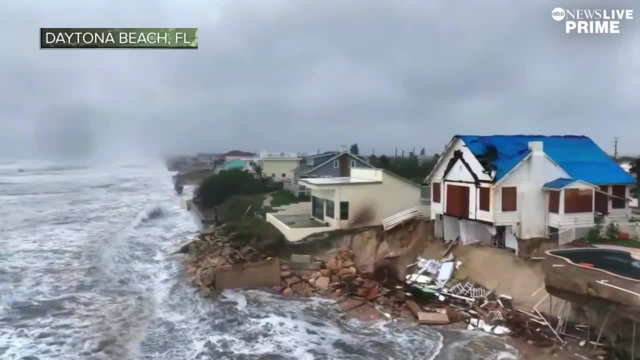 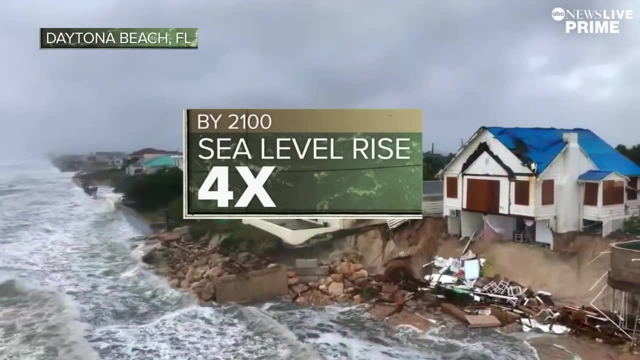 But the coastline has changed a lot in the last 18 years. Daytona Beach has seen a sea level rise of a foot in the last century, But by 2100, they'll see almost four times that. So warming our planet faster is correlated directly to that. 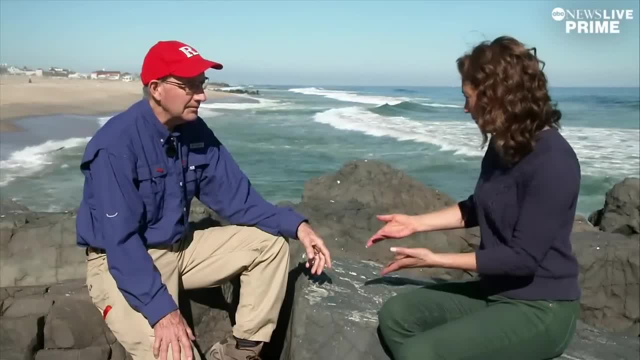 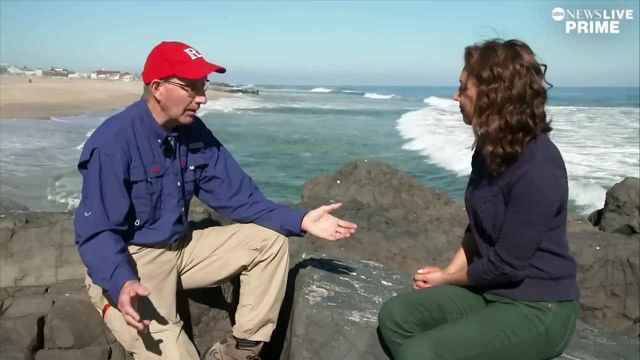 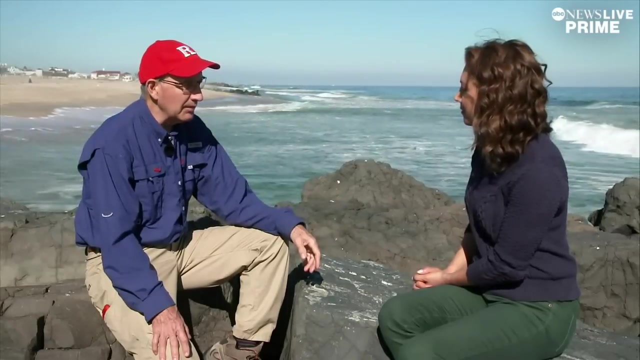 Is it correlated directly to the sea level rise and then erosion? Yes, Sea level is controlled by both the temperature of the water, so it is getting warmer, but also by the melting of the ice sheets and ice glaciers, And both of those contribute by putting more water into the oceans. 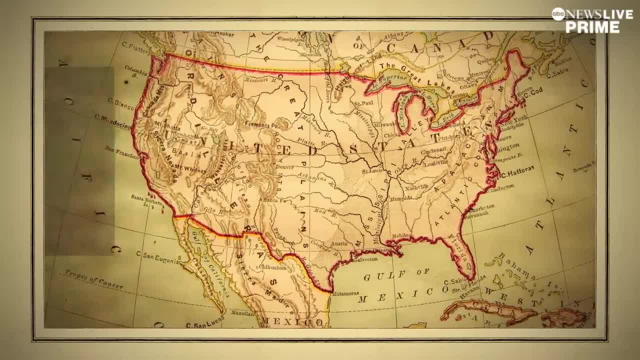 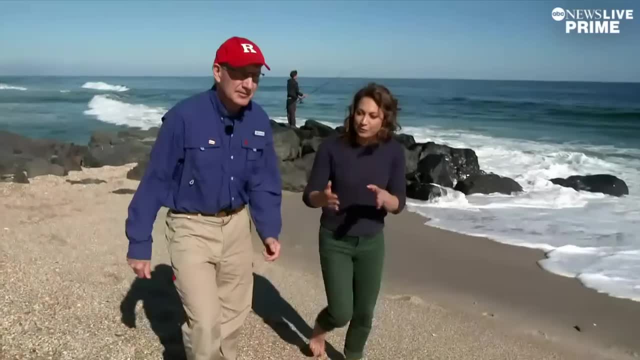 While sea level rise is not equal at every beach, the United States is projected to see an average of more than a foot in the next 30 years. That's more than it went up in the last century. If we see, okay, a foot by 2030, a foot of water, so what? 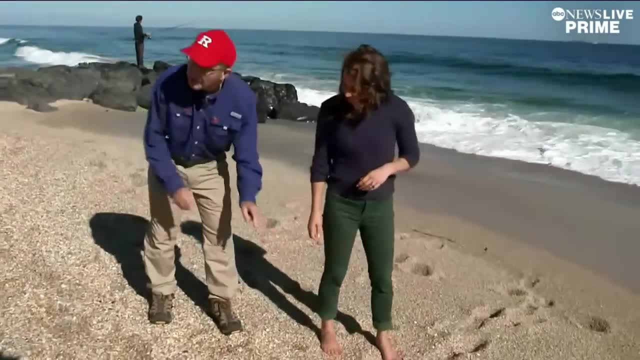 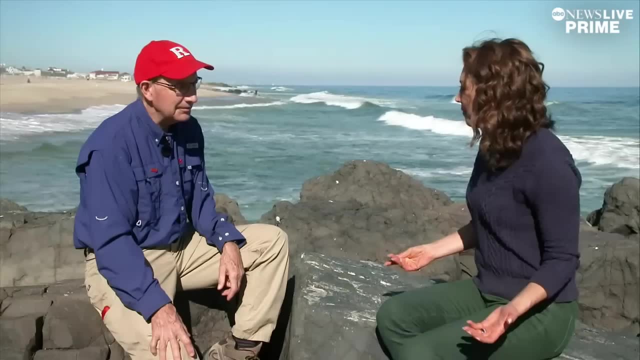 Remember, on a beach, if you have sea level rise of a foot, it's going to go 300 feet. in Rutgers, professor Ken Miller says it's simple: Higher water means more erosion. Why did we build right on the edge of the ocean? 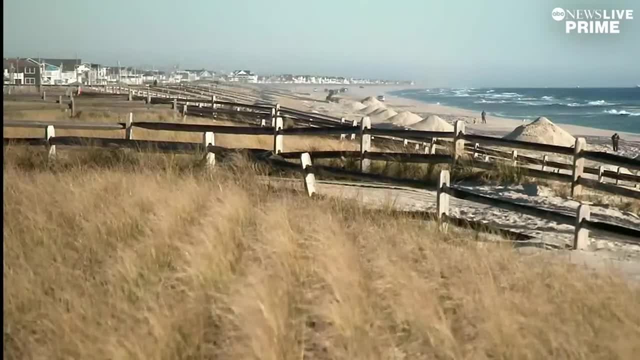 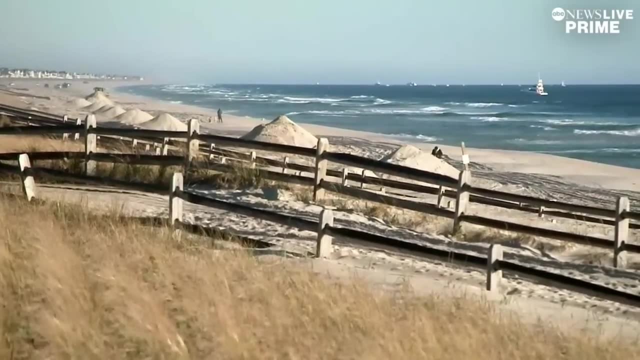 Who wouldn't want to live here? Most coastal communities survive on beach tourism And of course, without a beach you don't have tourism. Here- a costly man-made process called beach nourishment- It happens at almost every single beach that you see sand. 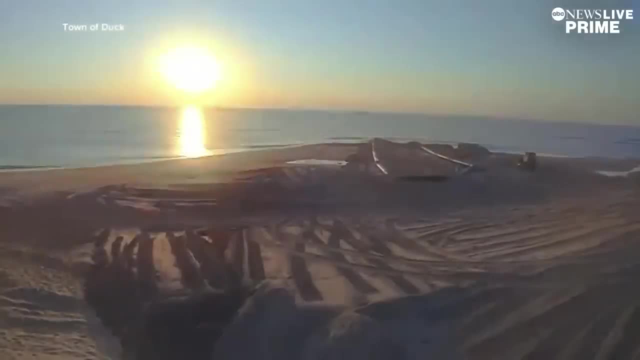 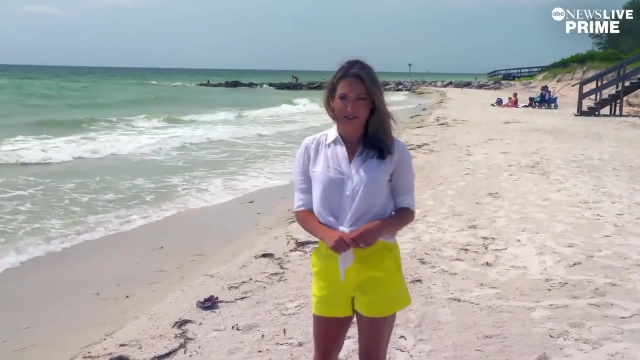 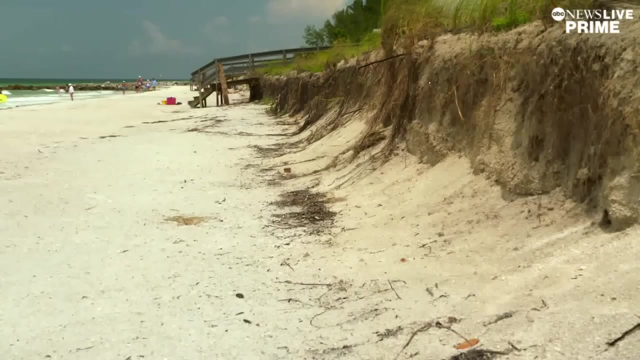 from Maine to the west coast of Florida and some parts of the Gulf Sand is taken from offshore and pulled onto the beach Sunset Beach. here this nourishment project will cost $12 million. The federal government spends $150 million every year to nourish the beaches around our nation. 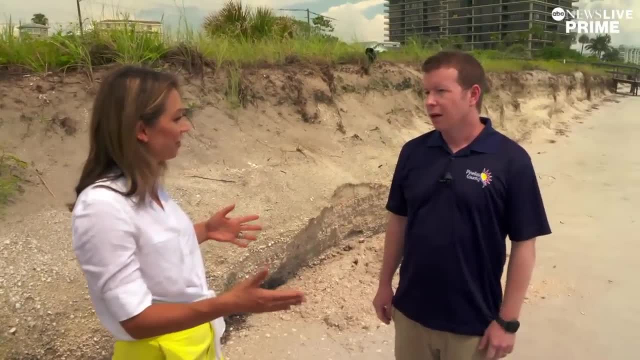 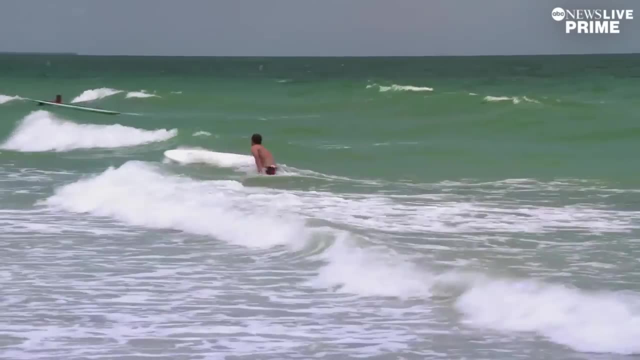 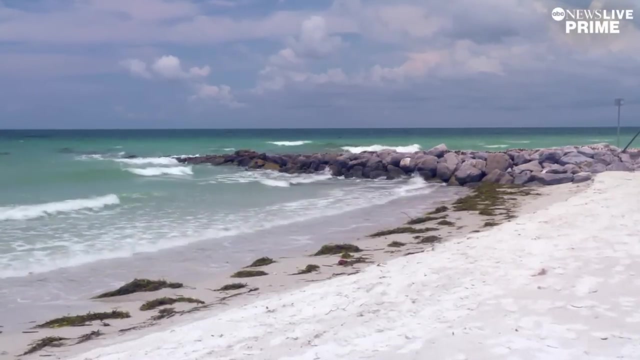 So within the last four or five years you've lost how much beach? Probably about 100, 120 feet or so. Pinellas County, Florida, has seen a half foot of sea level rise in the last 50 years every inch, making every wave more destructive. 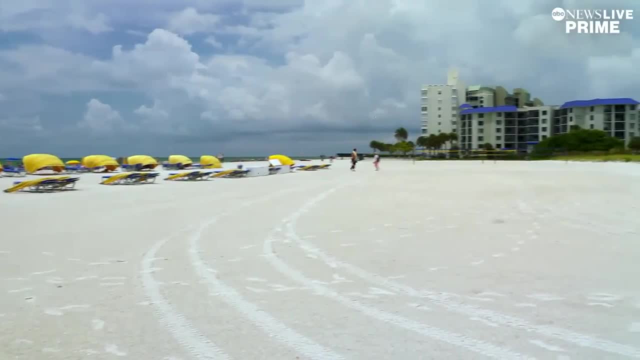 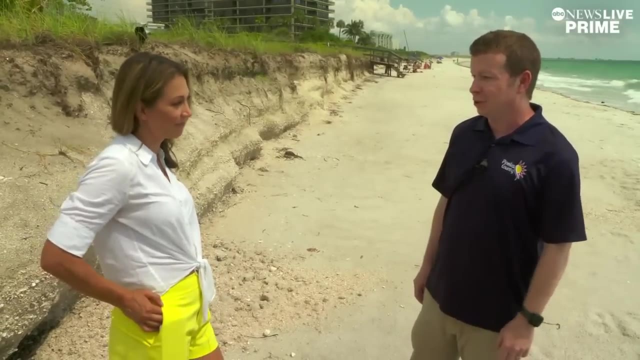 Now, if our beaches disappear, the economic impact would be devastating. These beaches are really Pinellas County's brand, and that brand is about a $9 billion economic engine that's driven by the 15 million tourists that come and visit us every year. 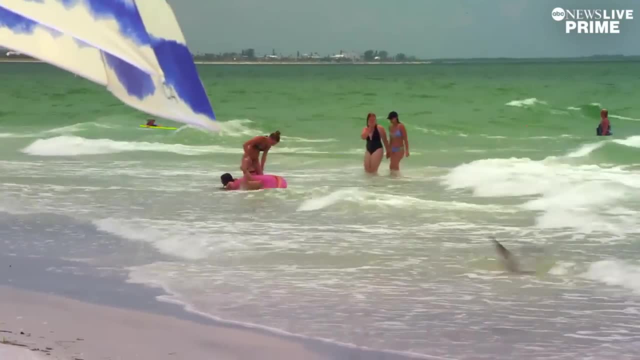 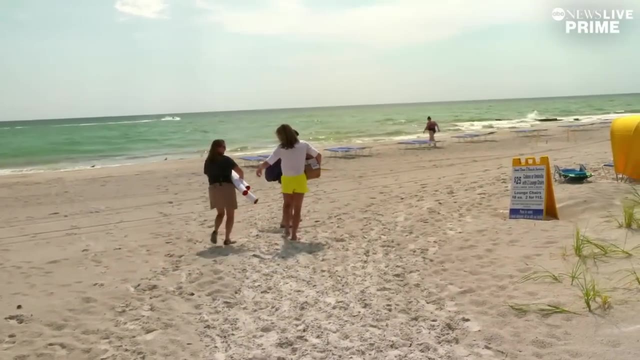 And that also supports 90,000 jobs. So there's a big emphasis on the return on investment. Okay, off we go. So you're carrying the actual sensor. I take it We tagged along with the USGS as they installed sensors to study our ever-changing coasts. 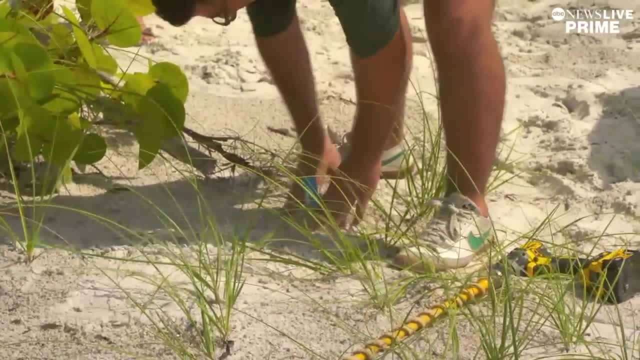 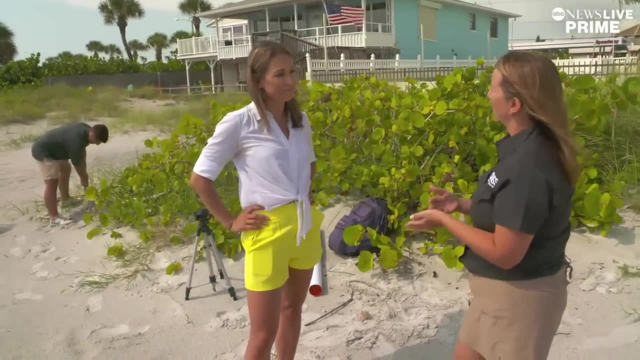 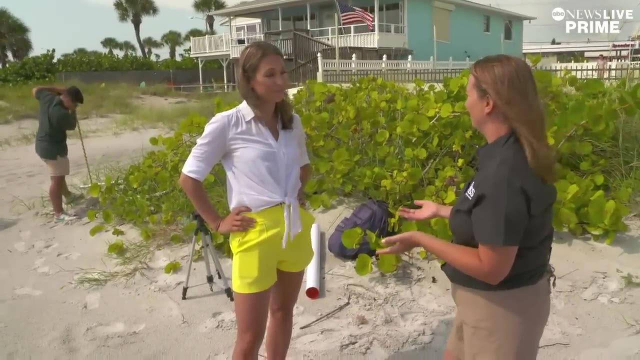 We can look at areas that have increased rates of sea level rise right now- relative sea level rise- like Louisiana. Well, Louisiana is a place where, over the last 100 years, we have shoreline measurements and we see that the long-term rate of shoreline change is 6 feet per year. 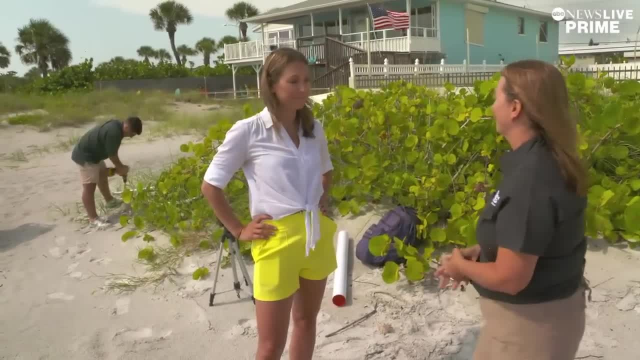 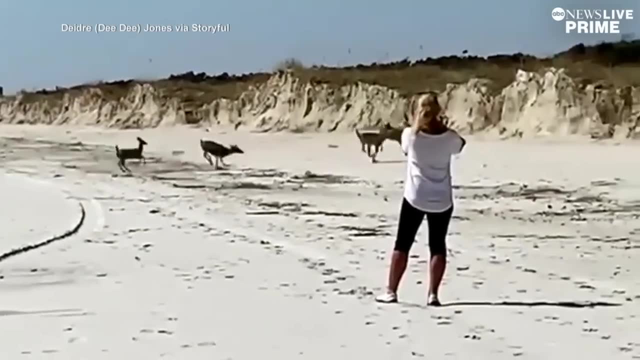 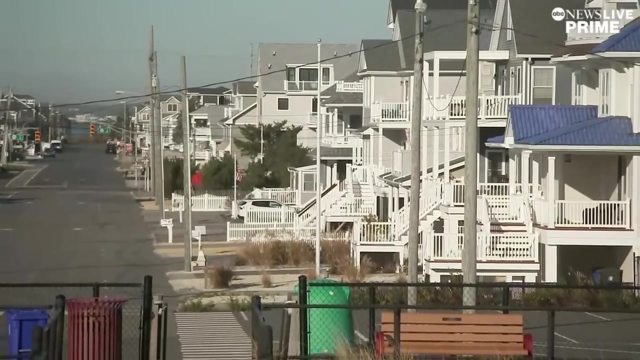 and we expect that to continue or increase as sea levels increase as well. Even after Ian, weakened erosion impacted the coast from South Carolina all the way up to Toms River, New Jersey, And remember that's a community that was devastated by Hurricane Sandy just a decade ago.